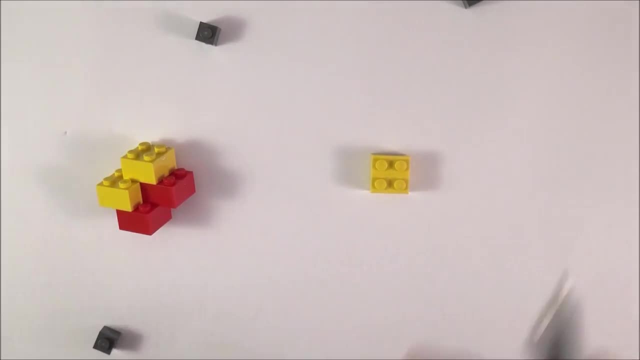 you have a positive charge and a positive charge over here. surely positive charges repel positive charges, so that when you try and put these close together they just want to repel. We know that. but then, if that's the case, how can we have a positive charge next to the positive charge here? 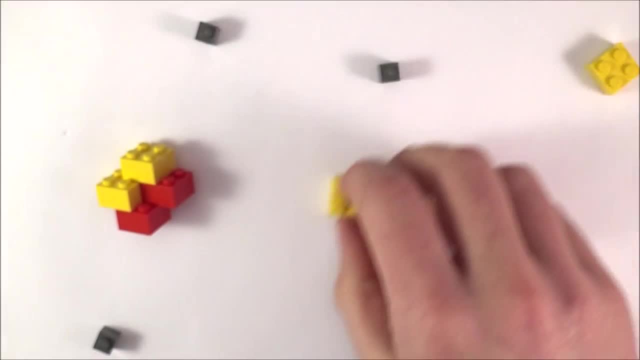 So what are the reasons? Well, basically, first of all, if we think about the electron orbiting around, maybe the central nucleus, and here we have maybe just a simple hydrogen atom, If this is moving around at any point, even though the force of attraction is inwards, if it's got a 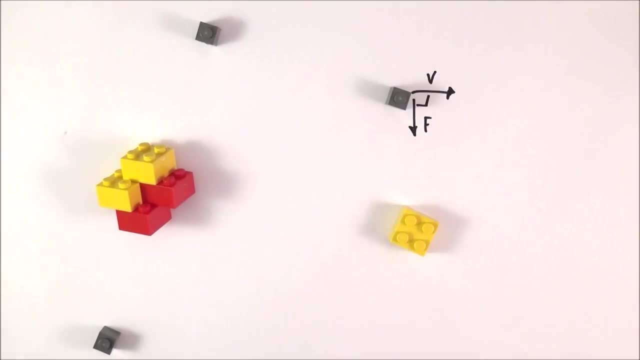 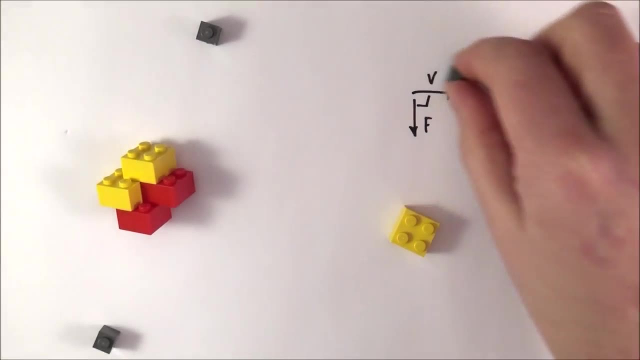 velocity in this direction because the force is at 90 degrees. that means this causes this to move with circular motion. So we think about just a nice particle. it's moving in circular motion, just a bit like the earth around the sun, and even though it's being attracted inwards, it's only 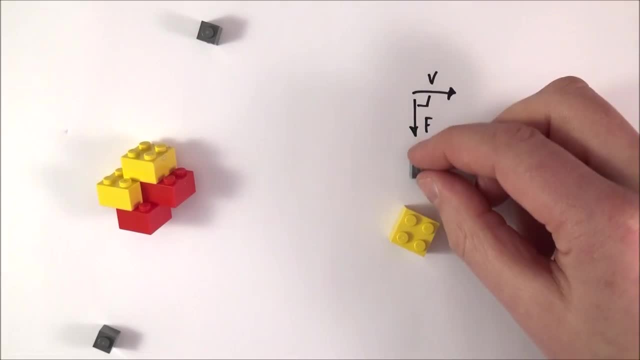 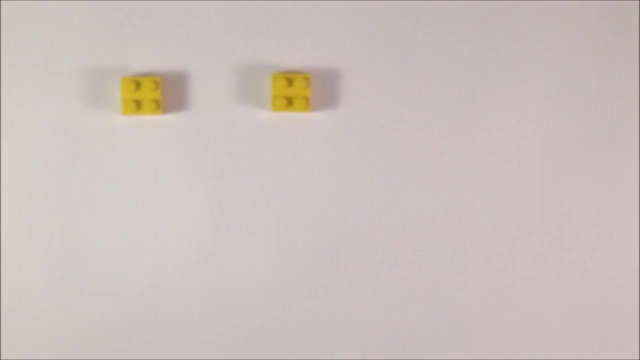 changing the direction, but not the velocity, and that's why the electrons actually don't go into the nucleus itself. The question, though, of why a proton can sit next to a proton is a bit more tricky, and that's what this video is really all about. So here I have a positive charge and another positive charge. 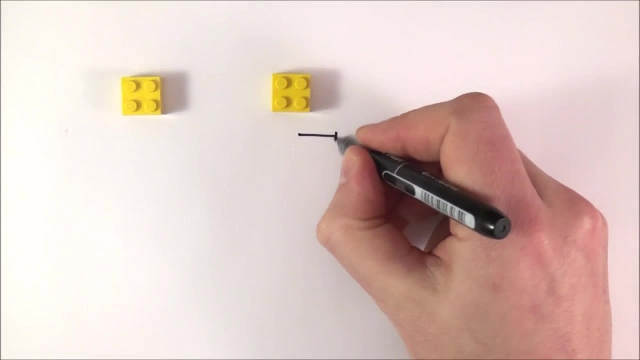 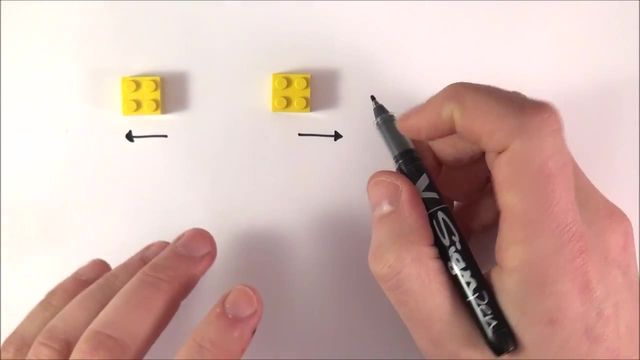 Now, at this time, if they're both positive, they're both going to feel a repulsive force, and I'm just going to put that in black. Now, this repulsive force is an electromagnetic force or an electrostatic force, and at this time you know these should be equal, but they're acting in opposite directions. 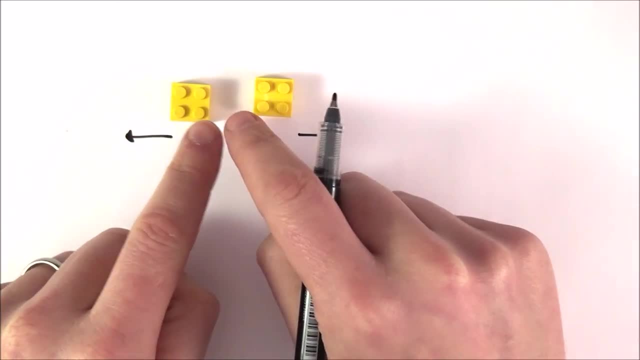 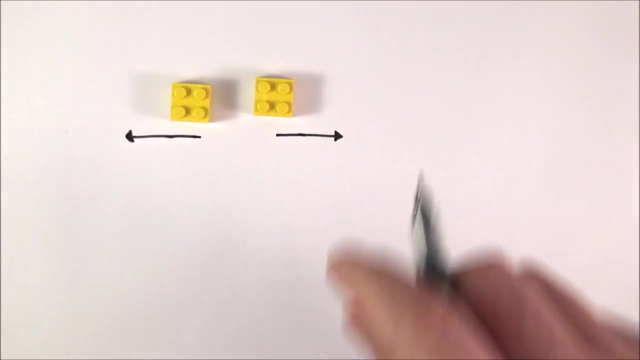 As you push them closer together because the distance between them gets shorter or smaller, that means the size of this electric repulsion gets bigger and bigger and bigger. Okay, so the closer they get together, the stronger they're trying to push apart. However, there's also a 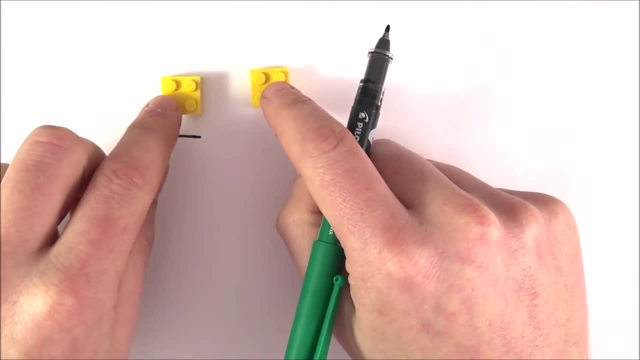 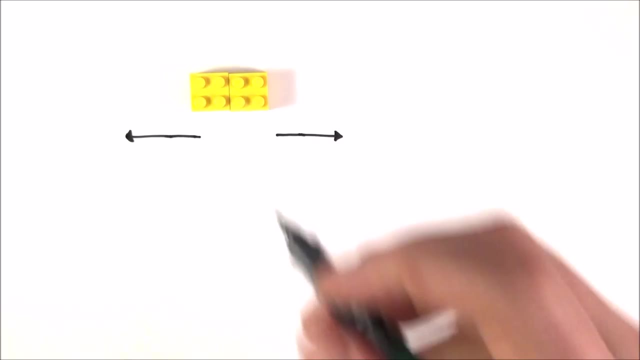 gravitational force, because these things have mass and when you put them closer together the force of attraction is going to be bigger and bigger and bigger. So maybe when they're very close together, gravity is pulling them together. but actually if I put the gravitational force here, that's it kind of. 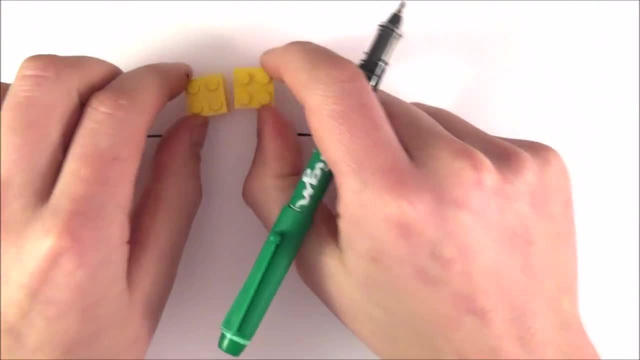 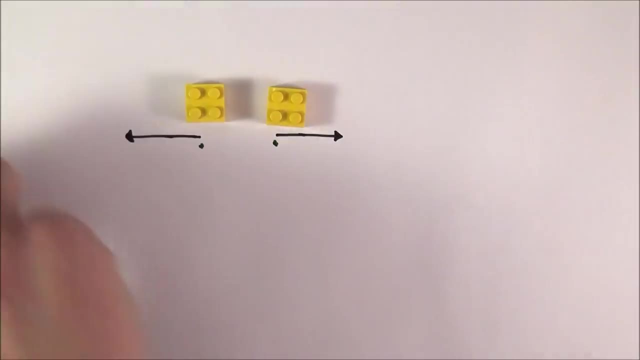 you can hardly see it, because the mass is so small. the gravitational force of attraction between these two particles is negligible, and that means there must be some other kind of force, Not the electrostatic force, not the gravitational, but there must be some other kind of really kind of. 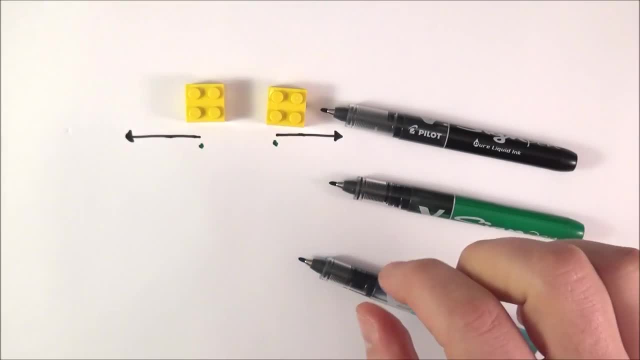 strong force that only acts at the scale of the nucleus, and indeed there is, and this force here is what we call the strong force, And it's this strong force here that when you, that only acts over a very short distance. So if I put the gravitational force here, and I put the gravitational 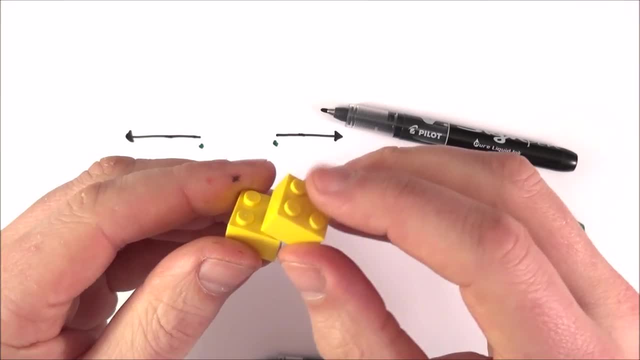 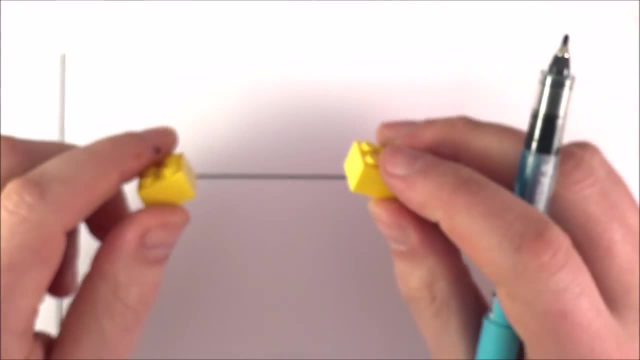 force at a very short distance, and when you have two things which are positive if you get them close enough, the strong force then will actually allow these two things to exist next to each other. Now, this strong force which acts between all the nucleons in a nucleus, basically it's carried. 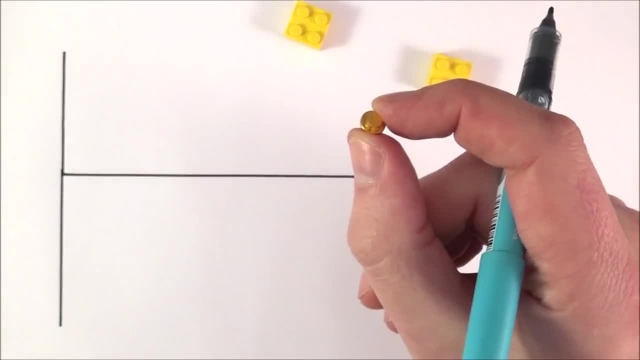 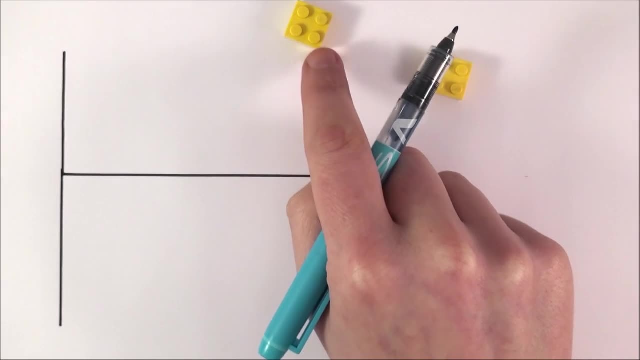 by something that we call a gluon. So this thing here is going to represent a gluon, and basically a gluon is what we call a boson, and this is what carries that strong force. Now, the thing is about these bosons is that they have a very, very short half-life, and that's because they 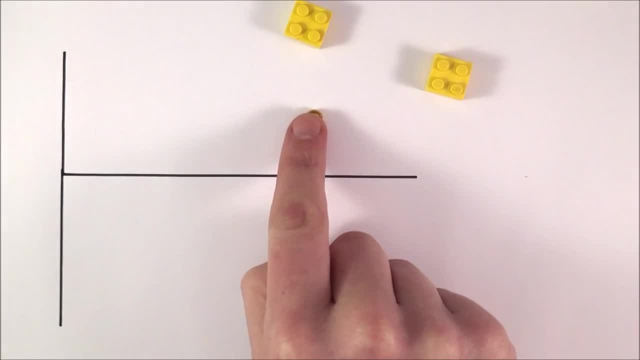 only exist for a very short amount of time, and that means even if they're traveling incredibly fast, you know, perhaps you know close to the speed of light, even if they travel at the speed of light, because they only exist for a very short amount of time, that means they can only transmit that. 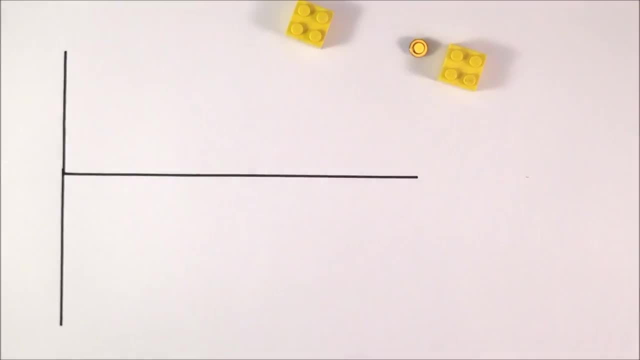 force over a very short distance And for that reason, if we maybe look at, maybe, the size of the force here, which is maybe positive or negative, when we go to a certain distance r away from you, know these two things. if they're quite far apart, the force has no impact and therefore, at a 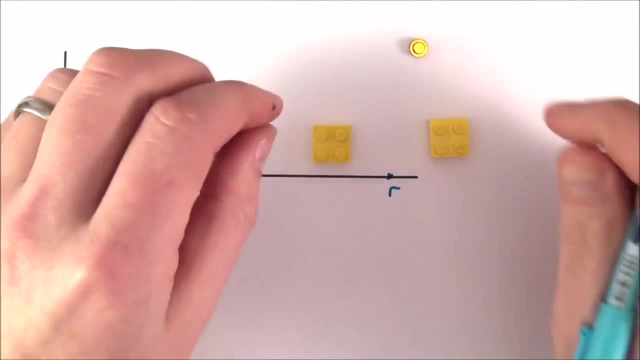 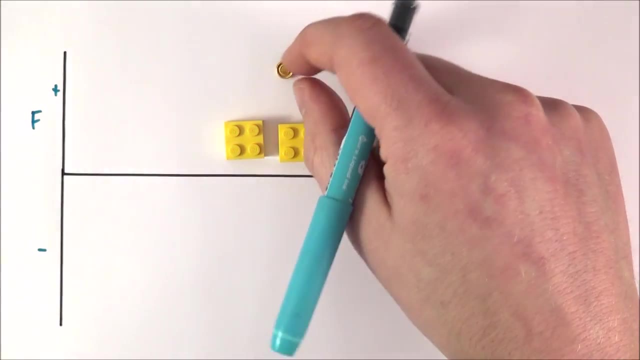 long distance away, these two things feel as though they're going to transmit that force. So if we look at, these two things feel no force. Now, when they get closer together, it's only then that we have this gluon which is kind of transmitting the force between them, and what we have then is an attractive 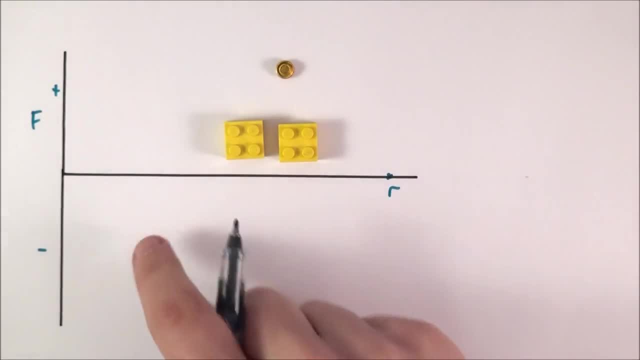 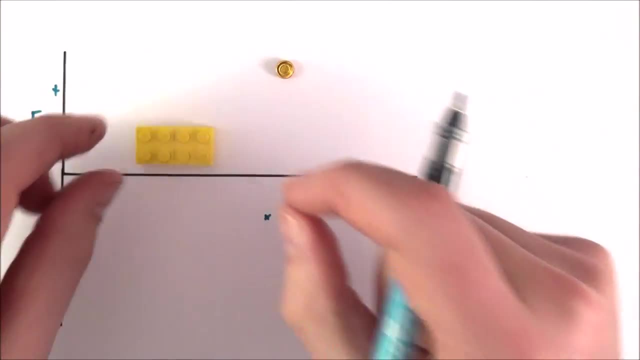 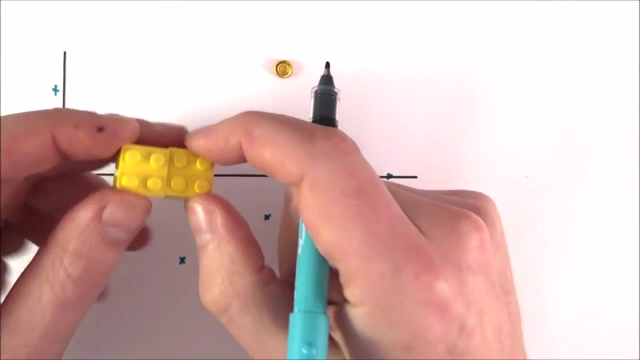 force. Now, an attractive force always has a negative symbol. so, basically, when these things are quite close, we have an attractive force. When they get to the perfect distance apart, that's when we have the maximum attractive force, and that keeps these things together. Now, at some point, though, if these try to get too close, you know, because if, at this point, 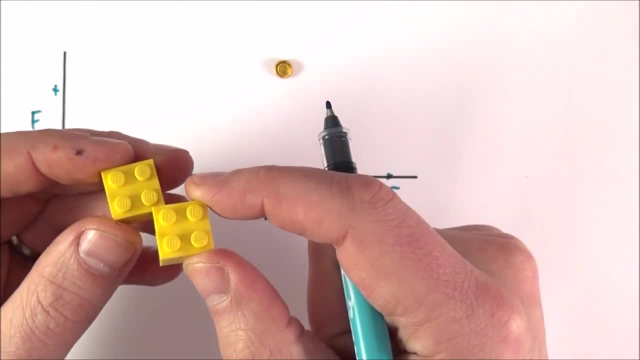 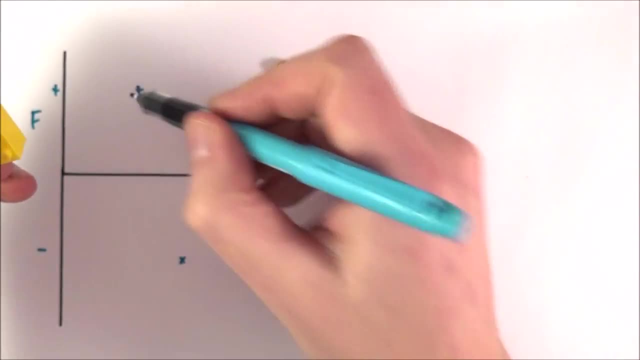 if there's a force kind of pulling in and pulling in, what's to actually stop them pulling into? you know, basically a singularity. well, when these two things get too close, that's when this force here becomes repulsive again, And what we actually see is we can look at this on the graph here.